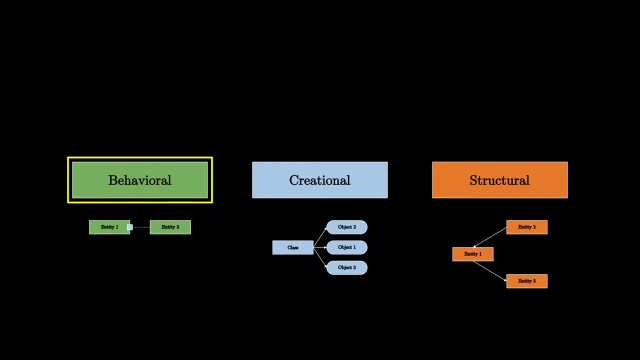 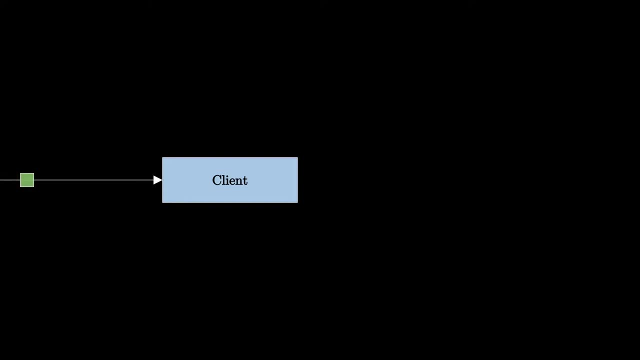 interaction between different components. To express that in a more visual way: if you got a class that is either receiving requests or is getting some data from an external component and you want to propagate that request or any event derived from it to other classes, then you may want to design your code so that you can easily add new receivers. 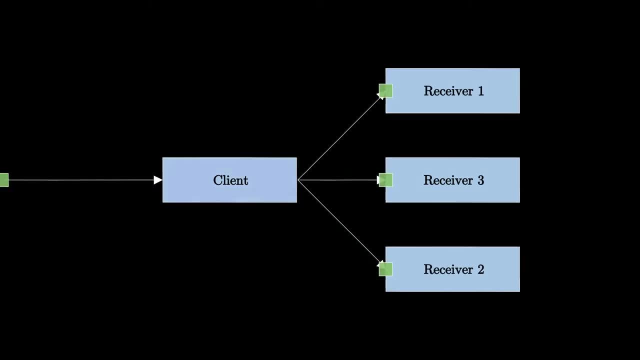 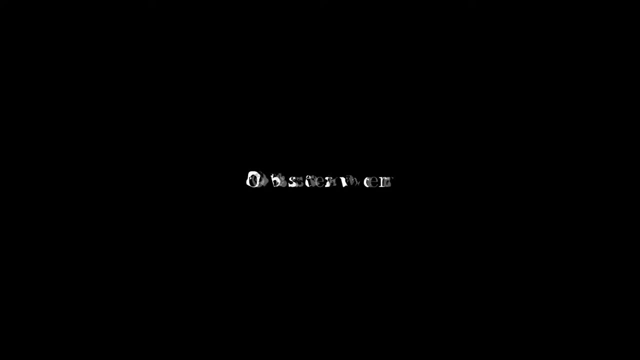 while keeping the components decoupled for better accessibility. In a nutshell, that's the role of behavioral design patterns. The first pattern we're going to talk about is called observer, and the reason you should know how it works is because it's related to other critical concepts that we see in the industry. 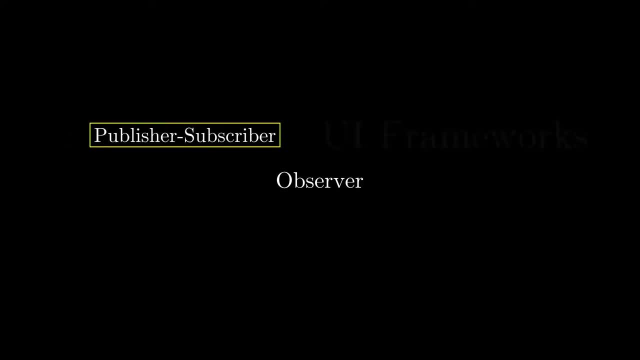 like publisher-subscriber pattern, UI frameworks, message use or even reactive programming that we're going to talk about in a future video. Now, the use case for which observer pattern has been created is the following: Let's suppose you got a class. let's call it subject. 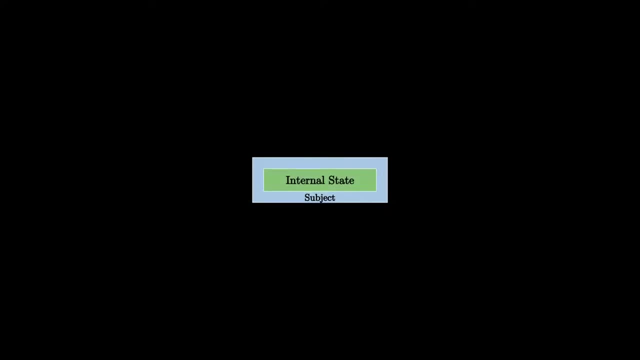 that contains an internal state which may change over time. We should see that internal state just as a bunch of private fields with some certain methods to be able to change them from the outside of the class. Now, whenever that state changes, you want other classes, let's call them observers. 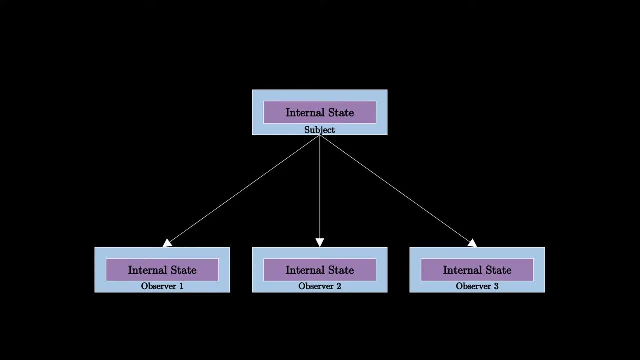 to be notified so that they can update their internal state or take any other action they want based on that event. There are two flavors or interaction models of the observer pattern. You need to pick a set of habit, cap options and bills when you're crafting your, when. 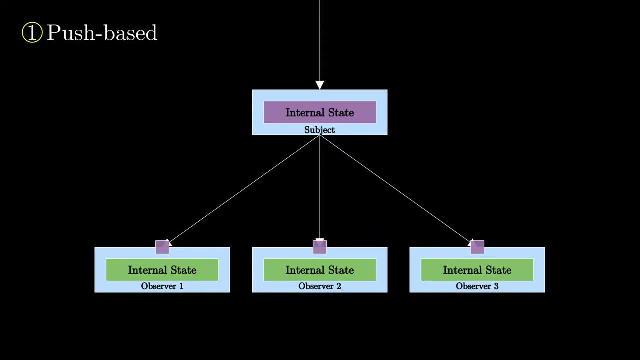 auditing. If you want to try those with consistent attributes, like commands, then this is the type of object pattern you're looking for, depending on your specific use case. The first flavor is Push based, which means that whenever the subject gets an update. 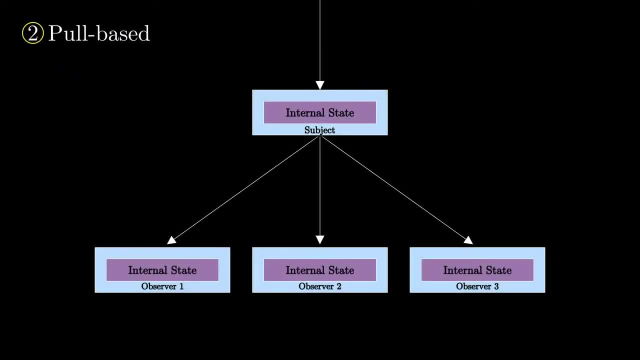 it will push that update to all the observers that are interested in its updates. In this case, the observers control what data they get from the subject. some of them may not be interested in the update at all and some of them may do something about it. 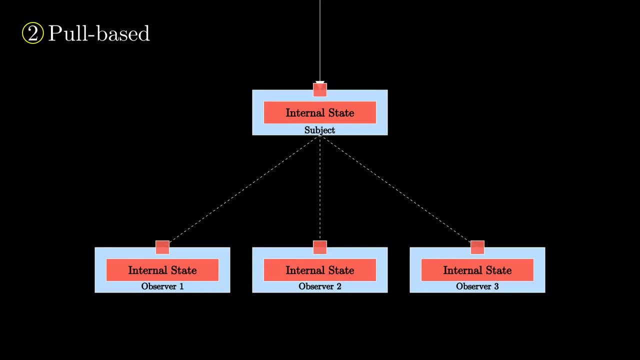 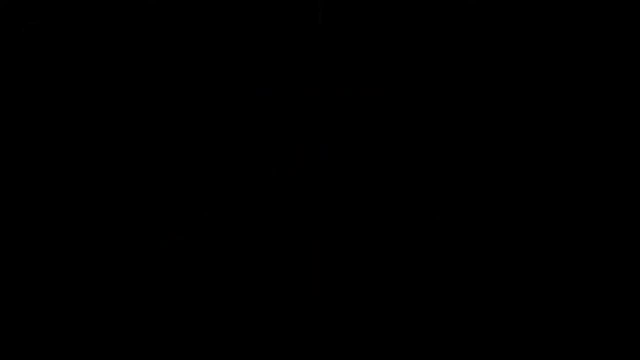 Both flavors have pros and cons, so you need to decide which flavor maximizes the vectors you need for your specific use case. Now let's take an example to see how the observer pattern works. Let's assume we have a class that is called database, which only stores a string field. 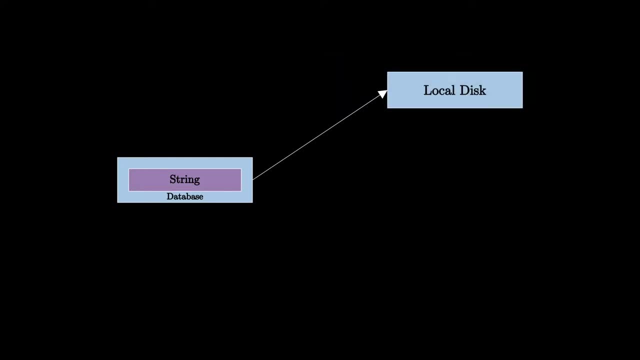 Whenever we change the value for that field, we want to store the update on the local disk, send an email and a slack notification with it. In this example, we're going to create both pull and push-based models, and we'll start with the push-based one. 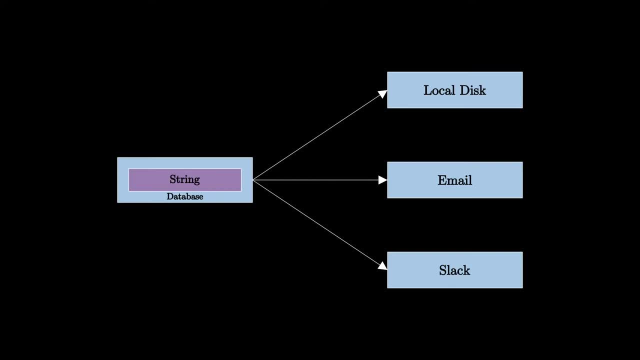 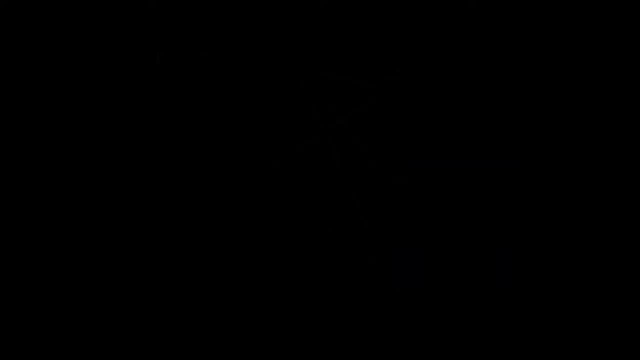 The first thing we need to do is to define the abstractions we need for the observer pattern, which are just two of them: the observer and the subject. For the observer, we can just create an interface with an update method that takes a string. 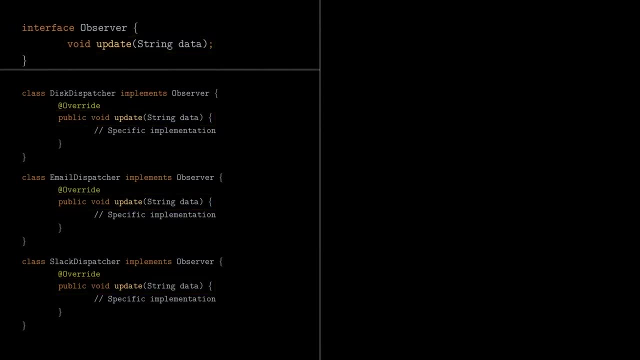 as a parameter. That's the actual update that we're interested in For the subject. we can create a base class that should provide the following functionalities: It should store the observers in an internal field in a list. in that case, It should provide an API to attach or detach observers dynamically. 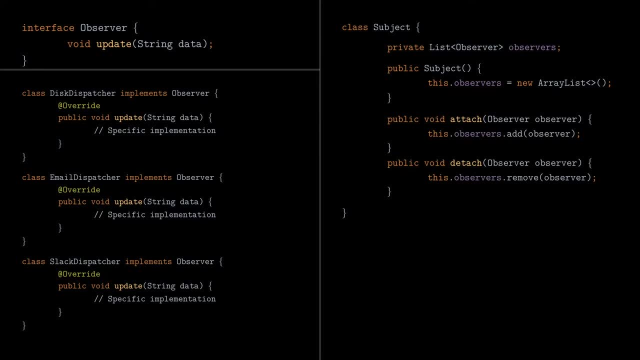 In other related contexts those methods may be called subscribe and unsubscribe, add or remove, link and unlink. They're essentially the exact same thing, as you'll see in this pattern. Now let's take a look at another example. And very important. it should provide a method that sends the notification to all the observers. 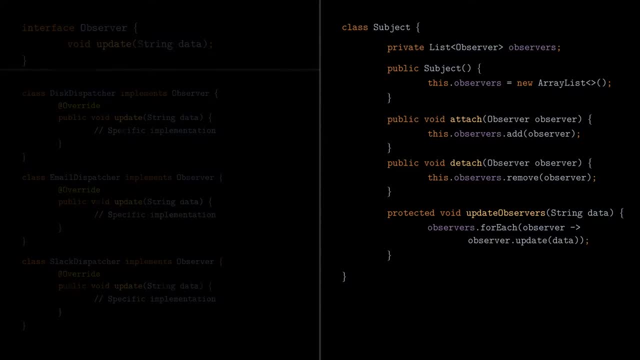 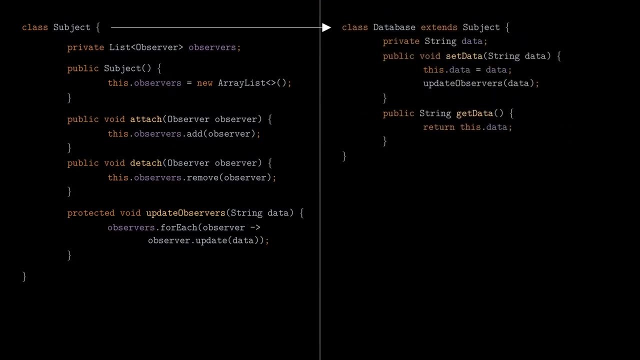 that are registered. This base class can be subclassed to implement specific logic. in our case to just manage that string field. Very important is to not forget to call the method in the base class that updates all. the observers Notice that from the subject we're pushing the data that has just been updated to all. 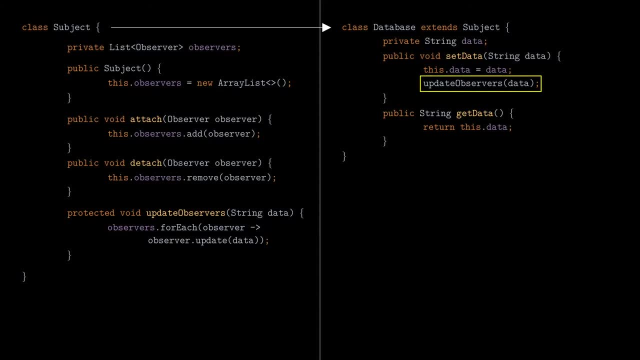 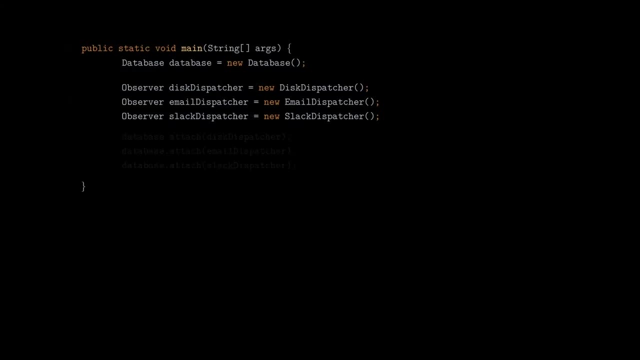 the observers. That's the idea of the push-based interaction model. The client will just create a subject and all the observers it needs, attach the observers to the subject and start changing the state of the subject to see the updates flowing around. Notice that we can dynamically add or remove the observers by just using the attach or. 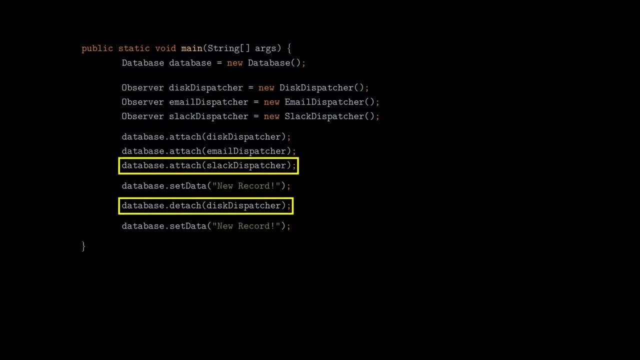 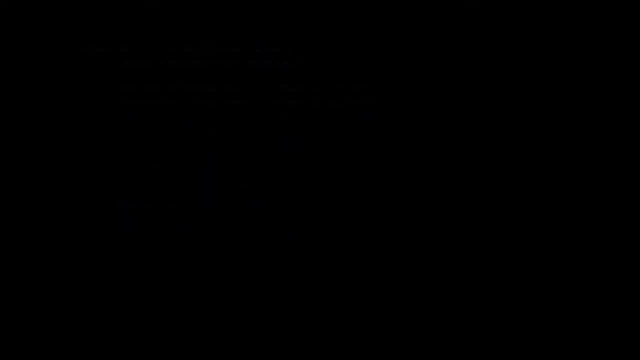 detach methods, which is something that really improves the extensibility of the code For the pull-based interaction model. we need to do some minor changes to the code. First, the observer abstraction needs to be converted to an abstract class instead of an interface. 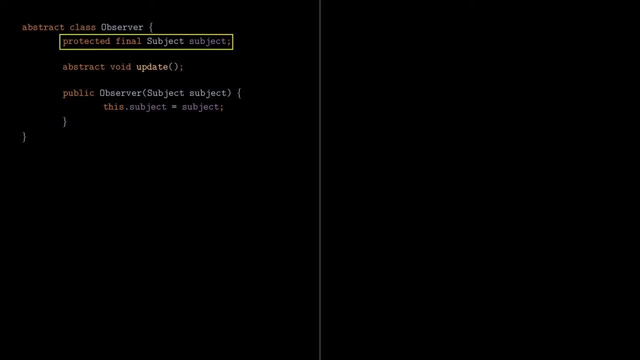 Since we need to store the object inside it to be able to pull the updated state out of it. The update method doesn't need a state parameter anymore, because now it acts just like a notification. When the object gets called, this is just a signal which marks that the subject state. 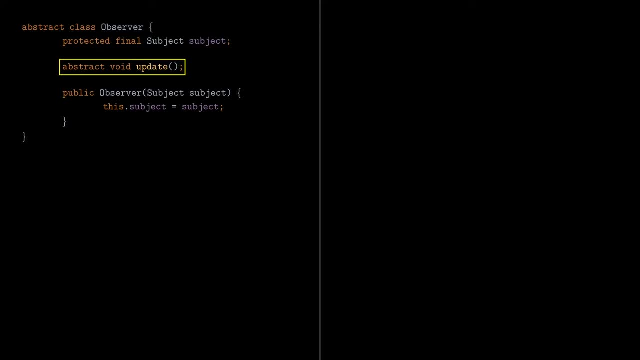 has been changed. The observer can ignore that or it can pull the state and do something with it. This decision belongs only to the observer. The subject abstraction needs to store the data payload because it needs to be accepted. We don't need to change the state of the observer. 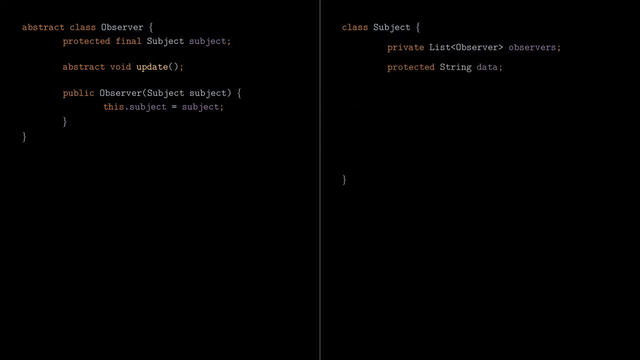 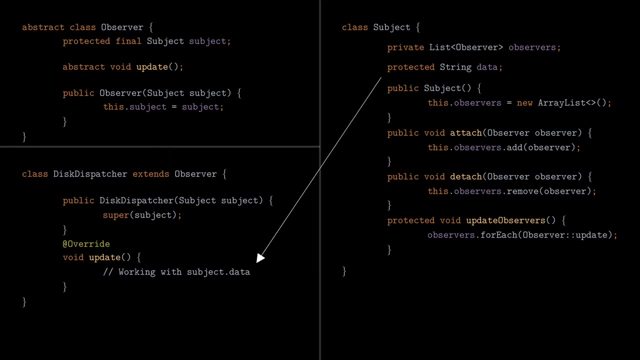 accessible from the observers, and of course those ones need to be updated accordingly. In a real scenario. you may also want to abstract the state as well, to improve the flexibility of the code even more. So that's pretty much all about the observer pattern. 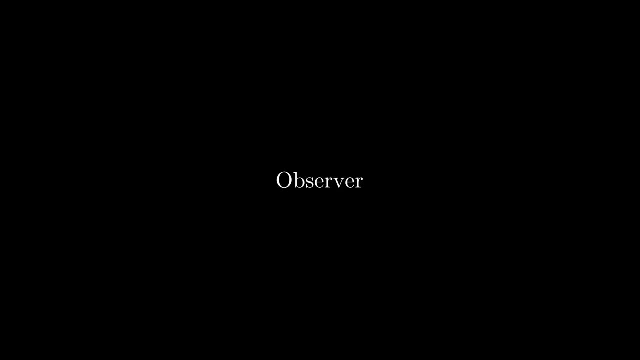 Let me know in the comments below what you think about it. Now we're gonna move to another behavioral pattern that has a slightly different approach. This one is called chain of responsibility, and I've seen it so many times in legacy codebases. The idea of that pattern is the following: 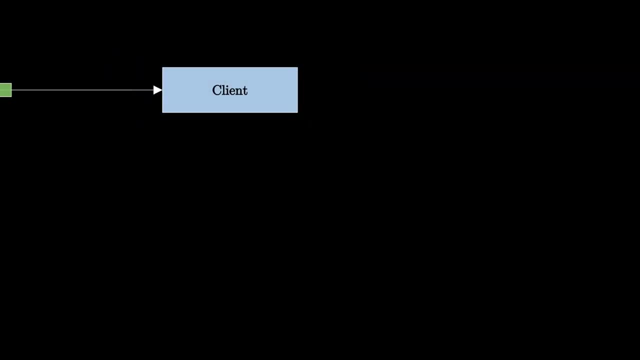 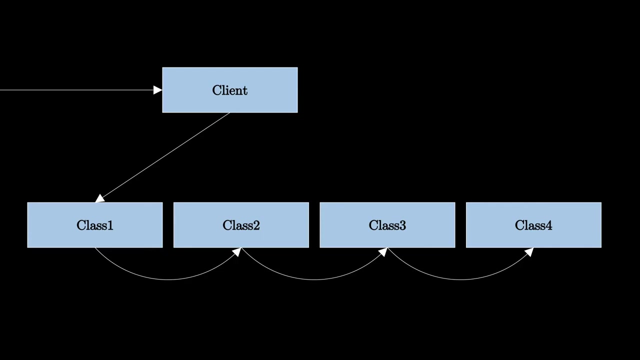 You've got a class- let's call it client, for example- that is receiving requests from another component. Each request needs to be processed, So to do that, the client passes the request to a processing pipeline which contains multiple classes that are chained together and each one of them is capable of processing that. 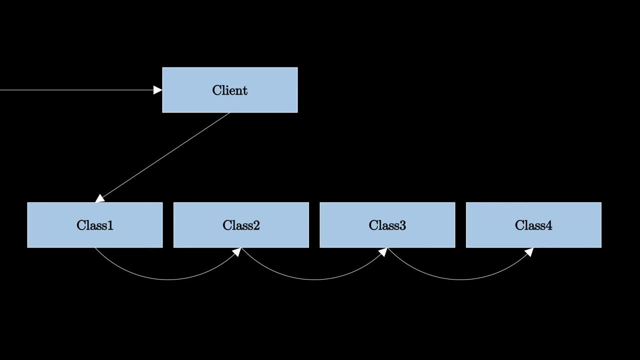 request. As you can see, the idea is simple: you get a request and then you pass it to that chain of classes in order to be processed. The way it works is that the client has a reference to the head of the chain and once. 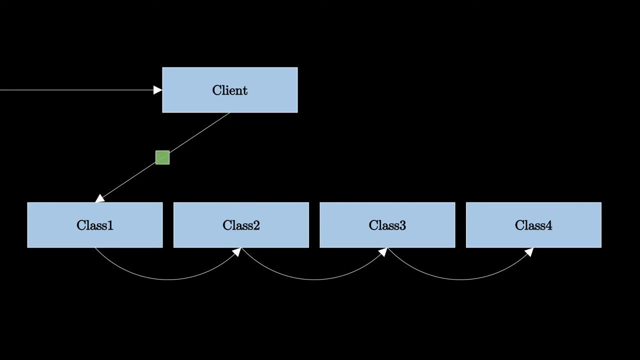 it receives a request, it gets dispatched to the first processing object, and this one should decide whether it is able to process the request or not. If it is, then the request will get processed. If it's not, it should pass the request to the next processing object. until there is 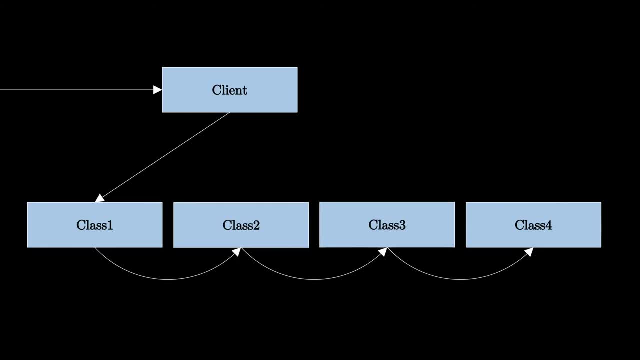 one able to process it. Now, of course, for this design to work, we need to make sure that for each request, there should be at least one processing object. So let's go ahead and see how it works. Let's go ahead and see how it works. 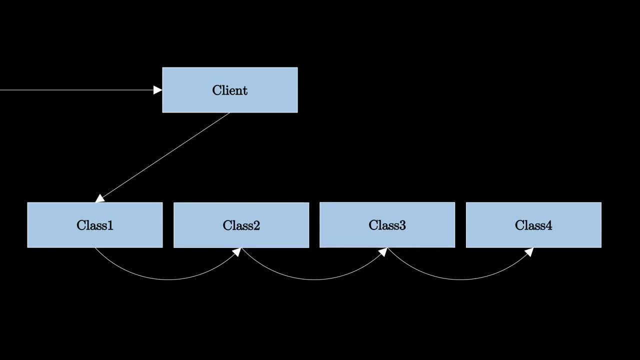 Let's see how it works. So let's say that we have one object in the chain that is able to process it. Otherwise, the request will just pass along the chain and it will not get processed at all. This is the only enforcement that we need to consider. 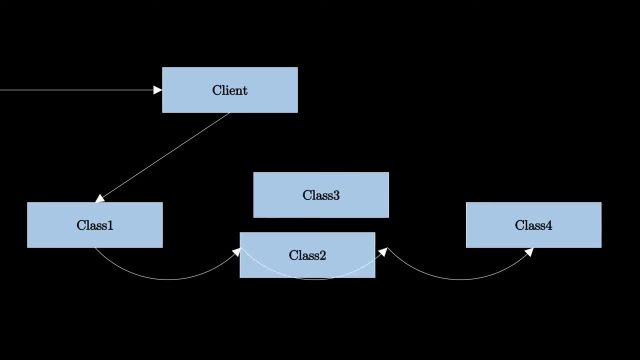 Now, depending on your specific use case, you may want to order the processing components of the chain so that you minimize the number of components that each request needs to pass through until it reaches the component that is able to process it. Now let's take a look on a conceptual sample code for that design pattern. 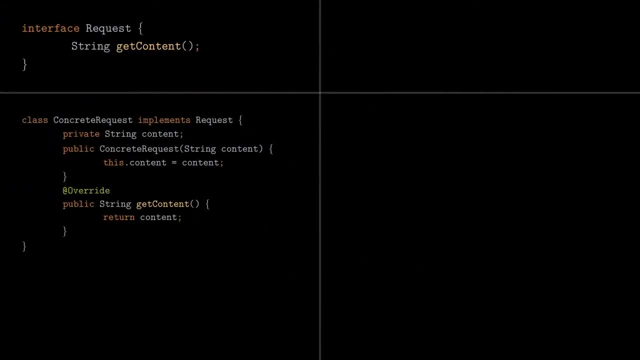 First, let's create an interface for the actual request that we're going to process. We can just assume that it has a string content. Now the handlers should also have an abstraction, which may look like that. We got a method that takes the request and processes it, and also one that tells whether 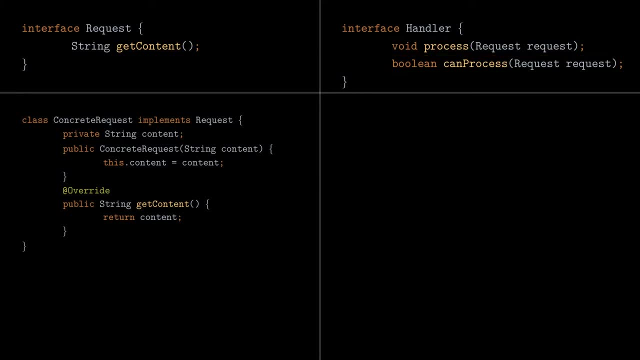 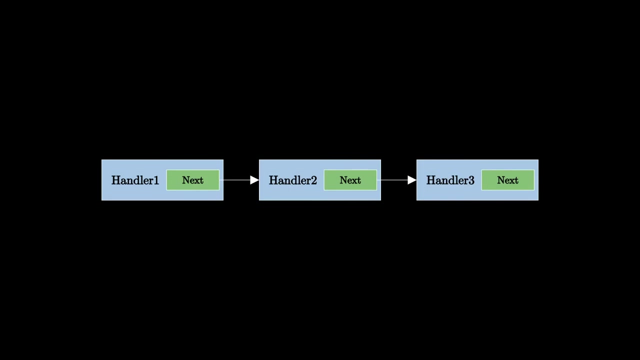 the handler is able to process the request or not. Of course, we need to create specific handlers which implement that interface, as we see in this example. Now, to create a chain of handlers, we have two options. We can either have each handler know which is the next handler in the chain, basically, 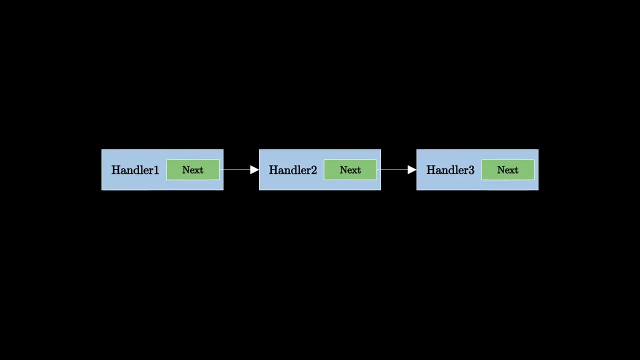 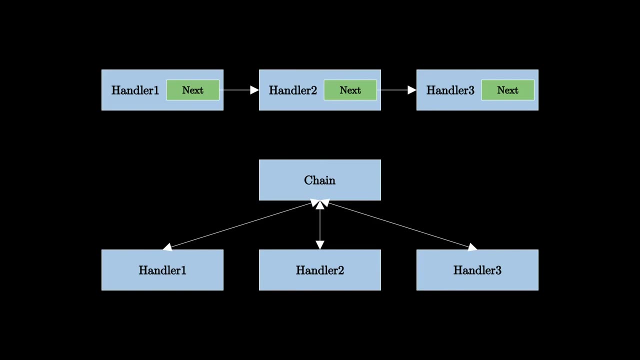 emulating a singly linked list, or we can have a class on top of the collection of handlers that manages the execution of the request through the chain. I personally believe that the last option would be a better one to implement that pattern, and we'll see why in a second, but first let's see how that kind of class would look like. 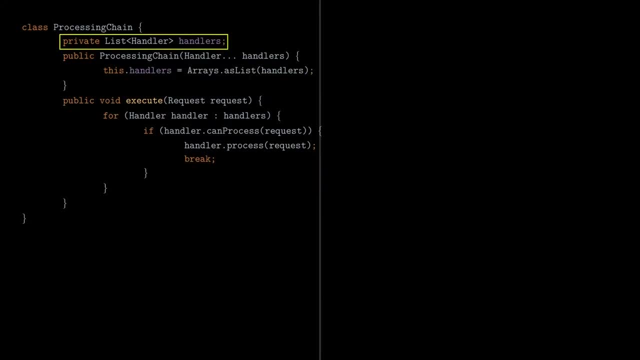 We can store the chain in any collection that preserves the insertion order of the elements, in that case an array list, and when we want to execute the request, we can just traverse the list and use the first handler that is able to process the request. 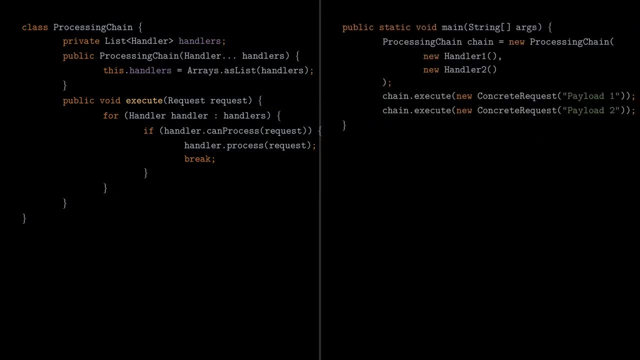 Simple and straightforward. The client will just create a processing chain with all the handler it needs and will just call execute to send the request. Now, the reason I like this option compared to the other one is because it's easier to order the handlers in the chain, which is something that you may need in most cases. 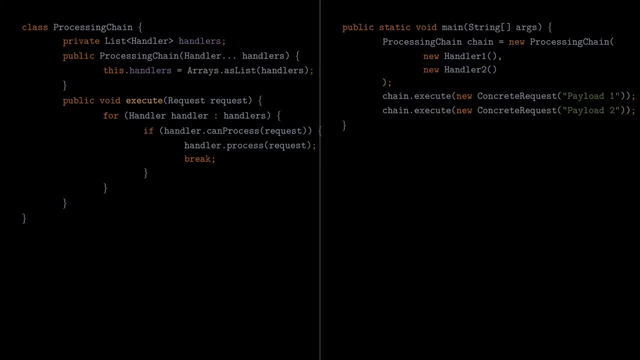 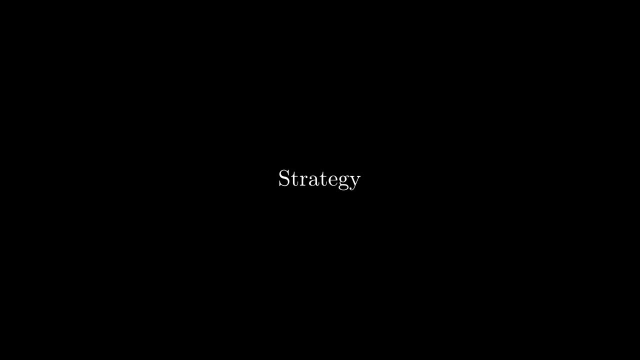 What do you think about that design pattern? Have you ever used it? Let me know in the comments below. The last behavioral design pattern we're gonna talk about is called strategy, and the whole idea around it is to hide different types of processing units under the same abstraction. 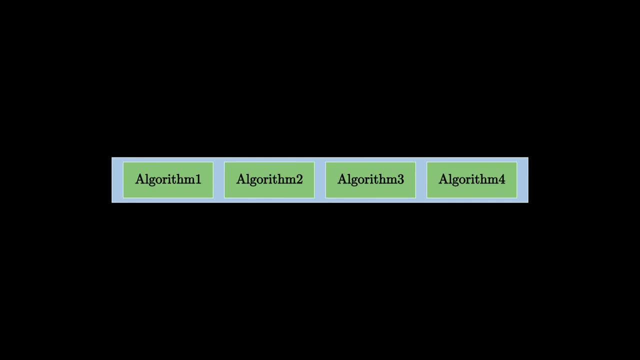 to be able to shift between them easily at runtime. In the Gang of Four those processing units are called algorithms or strategies, but they can be any type of logic that is likely to change over time, and they don't have side effects, so they are quite self-contained. 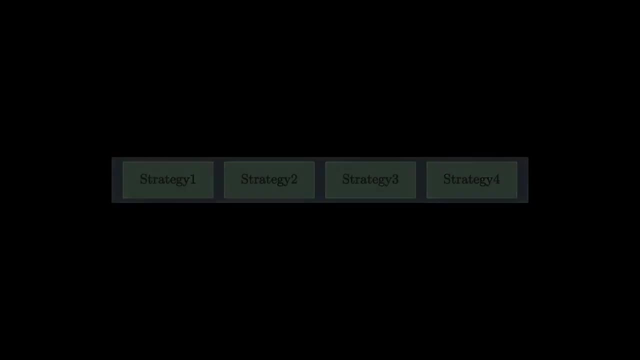 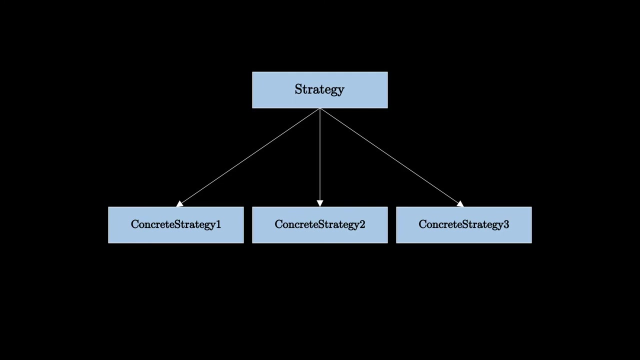 The architecture of that pattern is pretty straightforward: We get a strategy abstraction, which should usually provide a single method to execute the chosen strategy and, based upon that, we should have concrete strategies that implement their own processing logic. We should also have a place where we specify the selected strategy and use it to execute.